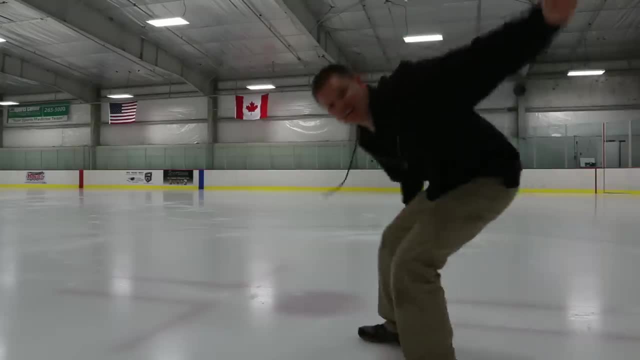 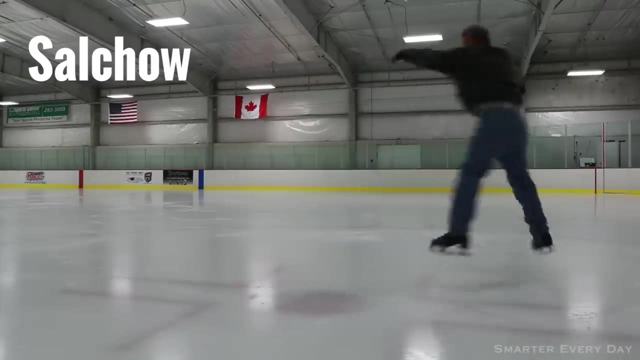 That's pretty cool. Alright, it's time to move on to jumps. Okay, Glenn's going to show us three of the main jumps in figure skating. Here's the waltz jump, The salchow And the flip. There's a gouge where you left the ice. 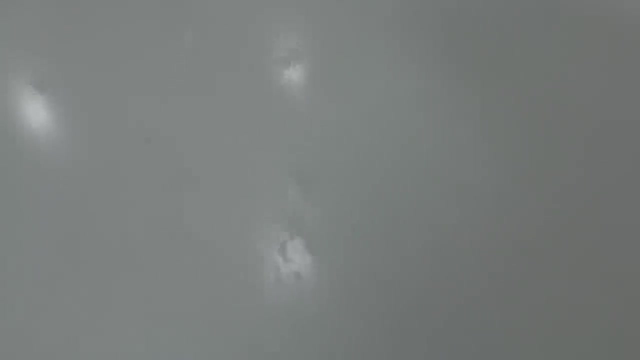 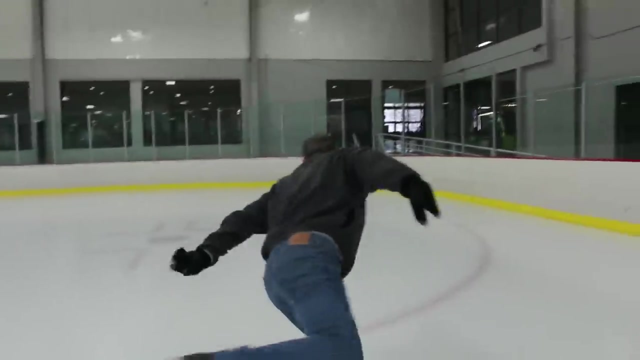 I pushed off my toe pick, Pushed off the toe pick, And then there's another gouge And I landed on my toe pick. Oh, And then I go down to my blade. So I'm pushing off the ice And I'm landing on the ice. 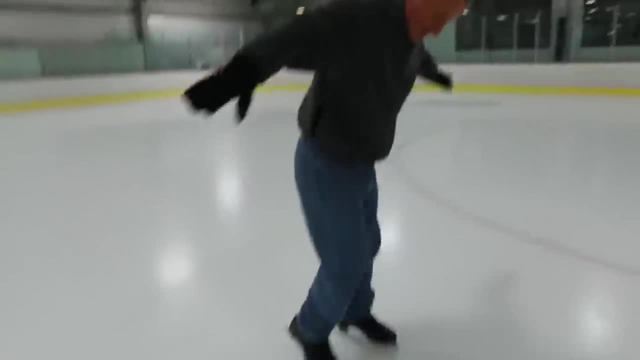 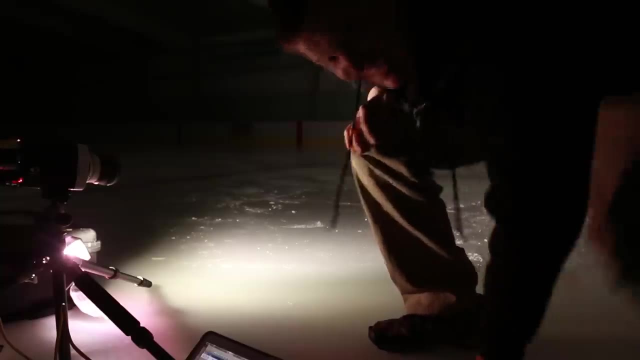 With the toe pick, With my toe hitting first and then my blade. Okay, Glenn's going to do a jump and he's going to land with his toe pick, which is how they always land. It adds stability. It's in the landing of these jumps where the design of the figure skates really start to show. 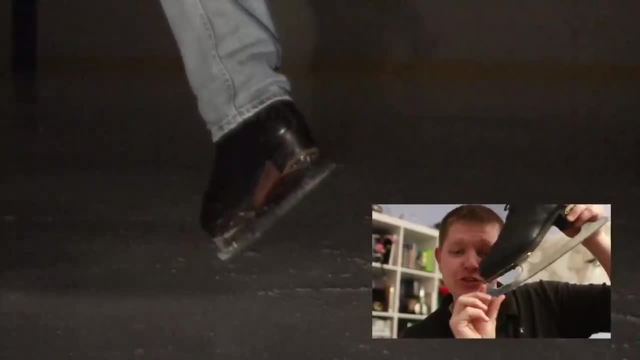 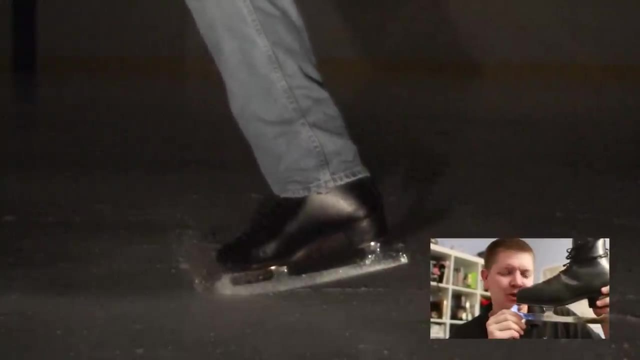 You can spike yourself down into the ice with the toe pick and then you slowly rock the blade down. In fact, the curvature of the bottom of the blade is called the rocker. After it's planted firmly on the ground, you'll notice it doesn't immediately move away. 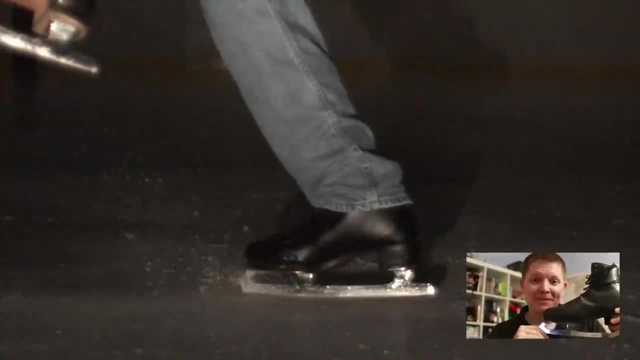 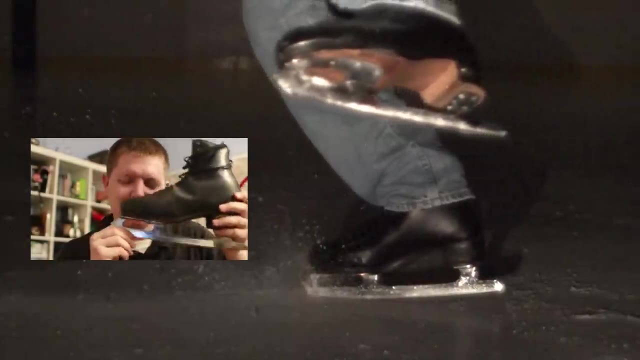 The skater imparts the momentum from his opposite leg back into his lower foot and then he moves. So it's a three-step process. Spike Plant Move- Interesting, But a question I have is that if the bottom is rounded, how do you sharpen a round blade? 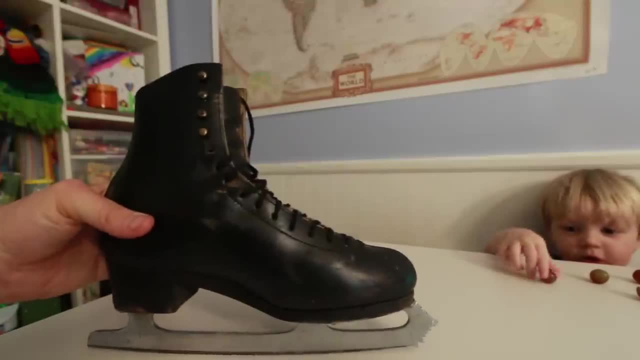 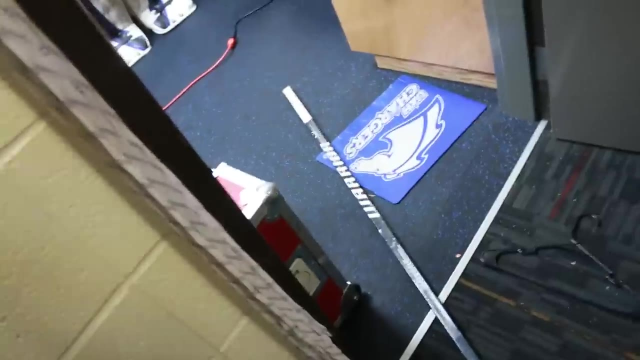 So this seems like a good opportunity to move from the figure skate to the hockey skate. So let's meet my friend Nick, who's the director of hockey operations at UAH. So you're going to show me, I'm sorry, Second time. 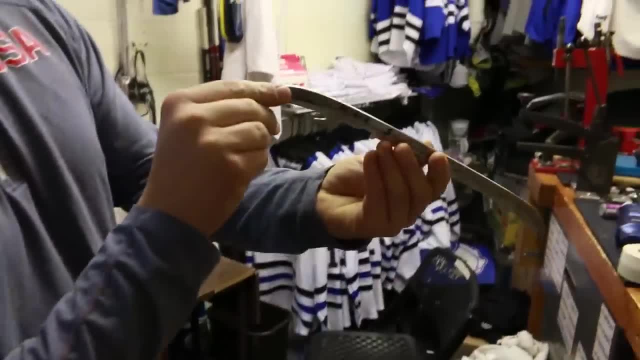 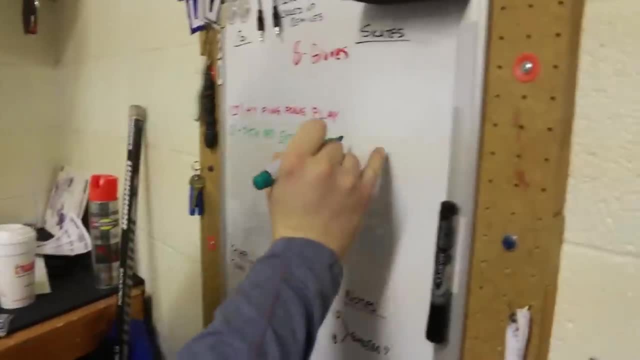 Sorry, dude, Show me the blade. How does this work? So the blades here. if you look, it's two separate edges, So I'll draw up here for you. Okay, Blade actually. So this is the cross section. Looks like that. 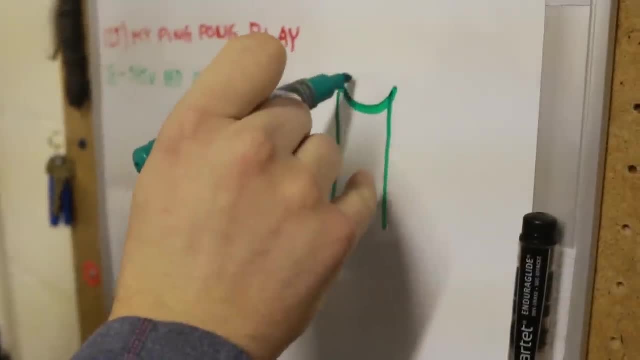 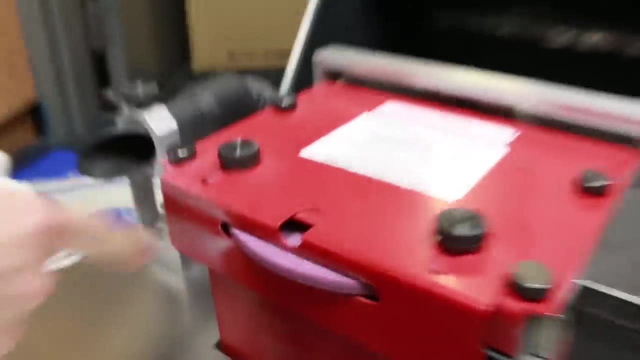 No way. A lot of people think it looks like that, but it's actually there's a hollow in here, Really, Yup, Can we see the sharpener? Yeah, I like the name Blade master. This is the wheel which actually sharpens the skate. 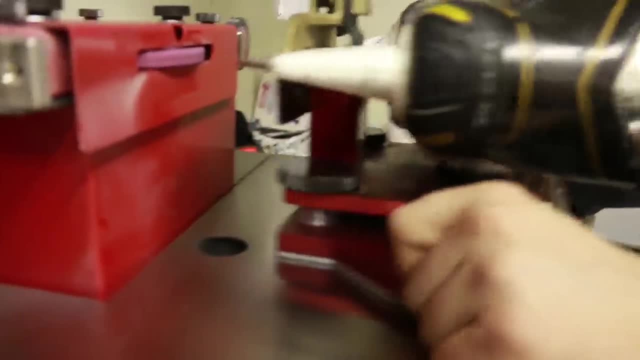 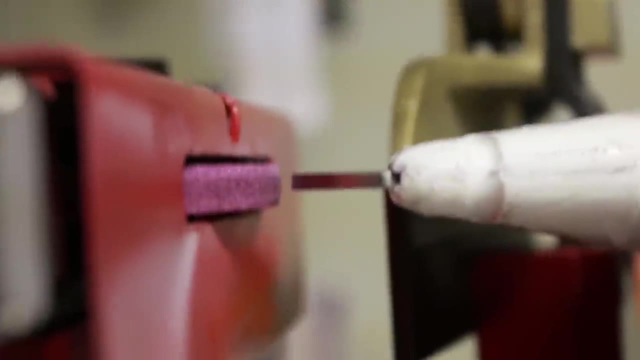 How do you hold the blade up there? Is this a sled or something? Slider? Everybody's got their own little nickname for it. Okay, And so then, if the wheel were turning, you would bring that in there. Let me focus, Okay. 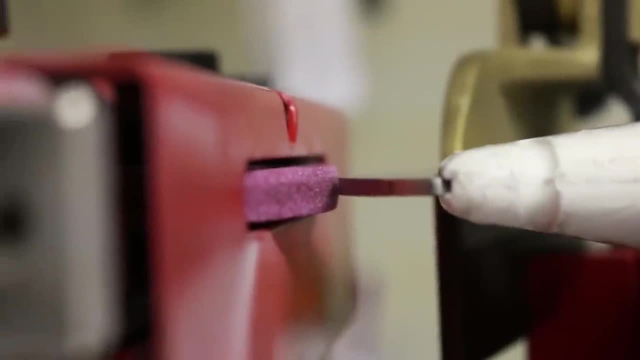 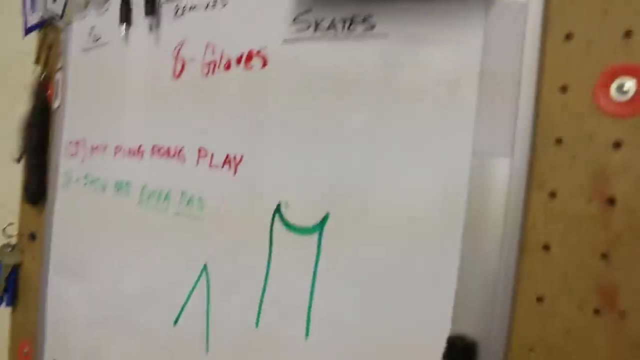 I can see that curvature that you're talking about. Can you go closer, if you would, to the wheel? So that's the radius of the skate: Three eighths, half five eighths. I'm not sure I understand. You're saying this hollow right here. 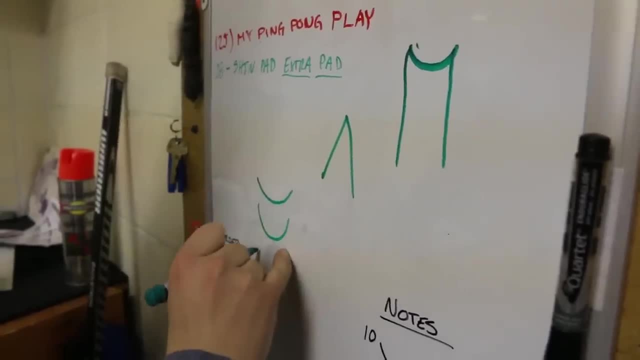 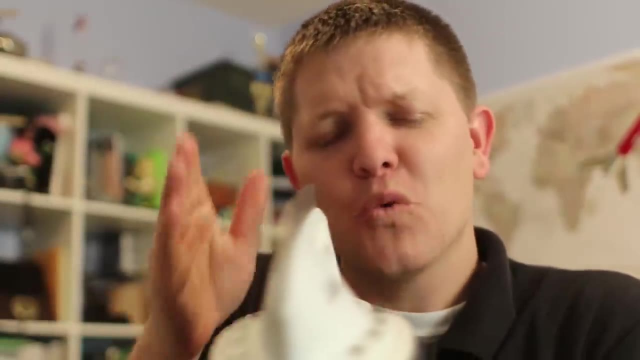 Yeah, Some of them will look like that. Some of them will look like that. Some of them will look like that. This is completely eye opening to me. I had no idea that ice skates had two different working edges. So why would a player prefer a deeper hollow versus a shallower one? 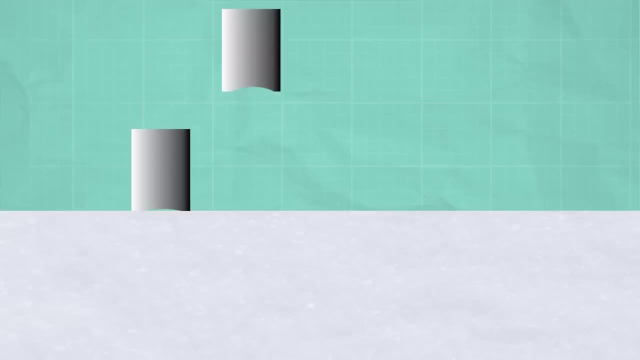 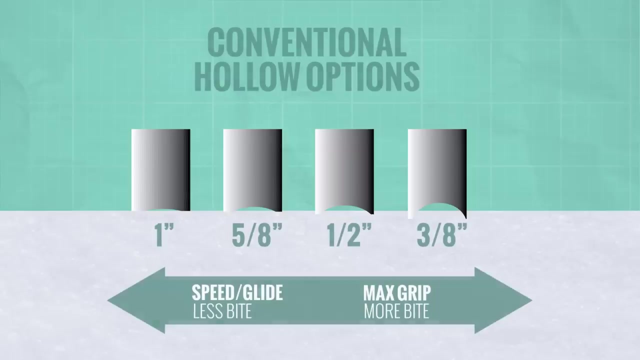 Well, think about it. If you have a shallow hollow, you're able to sit on top of the ice and glide very easily. So this is very good for speed, But if you have a deep hollow, your points are going to cut down into the ice and plow. 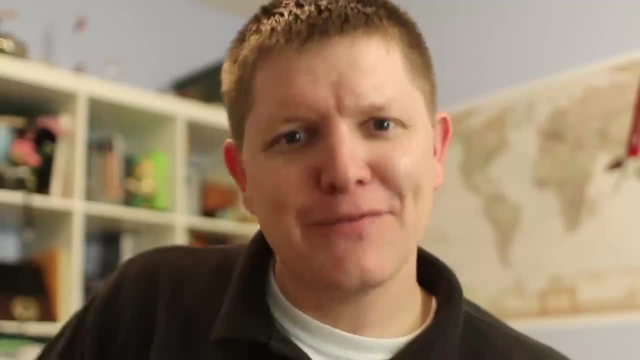 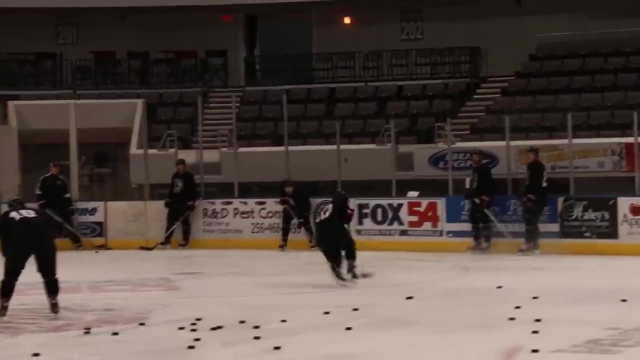 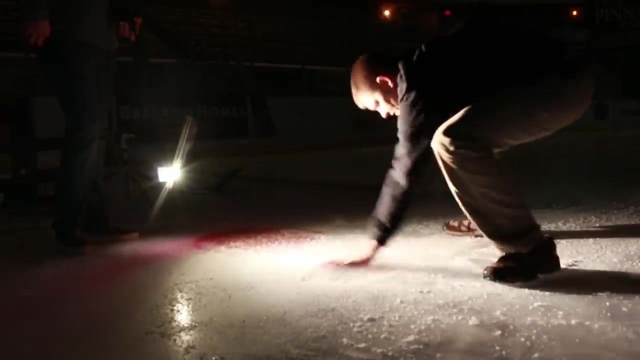 So you'll go a lot slower. However, you'll get much better grip, And if there's one thing a hockey player needs, it's good grip. Have you ever seen them stop and change directions? So I asked a couple of hockey players to show me how this double edge is used to stop on ice. 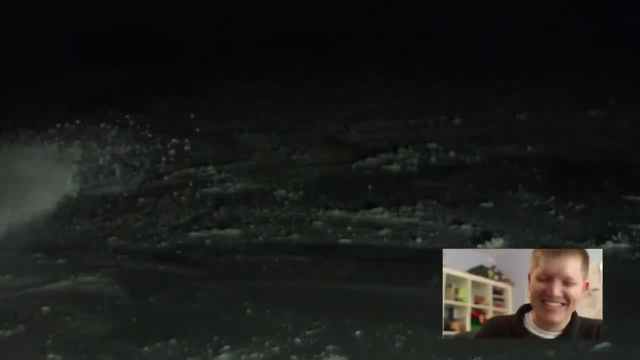 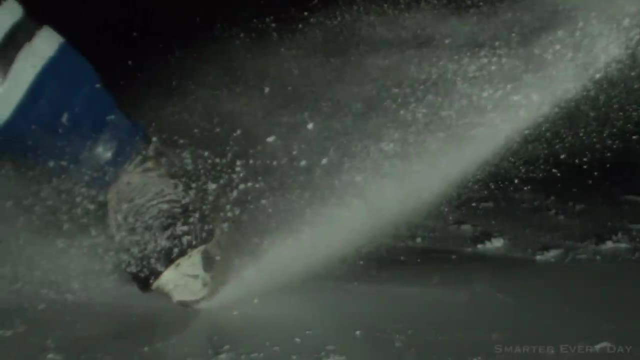 Behold the awesomeness of physics, Isn't that crazy? Look at what he's doing. He's controlling that edge and scratching the top layer of ice off, But he's doing it in such a way that it's converting that sheer energy into power, which he's using to decelerate. 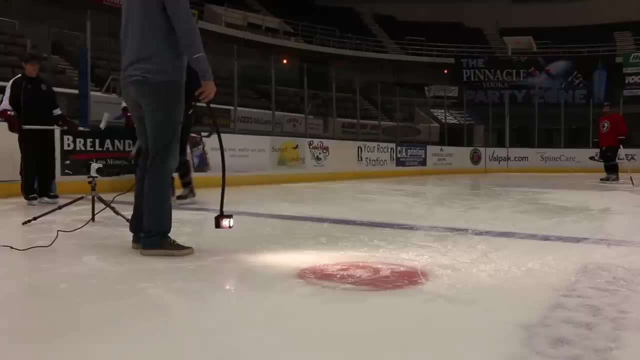 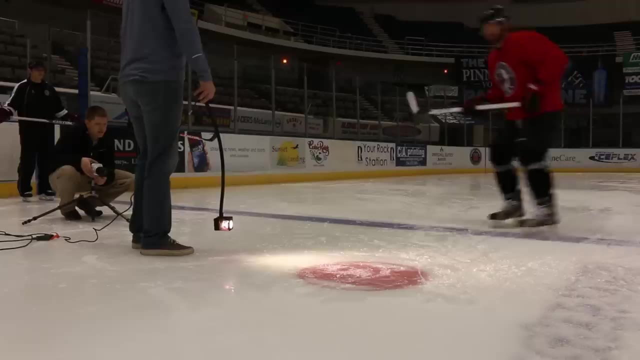 Some people want to believe that hockey players are just dumb brutes, But I'm not buying it. I told this player I wanted him to stop on a very specific spot on the ice so I could zoom in with the Phantom and catch the ice spray. 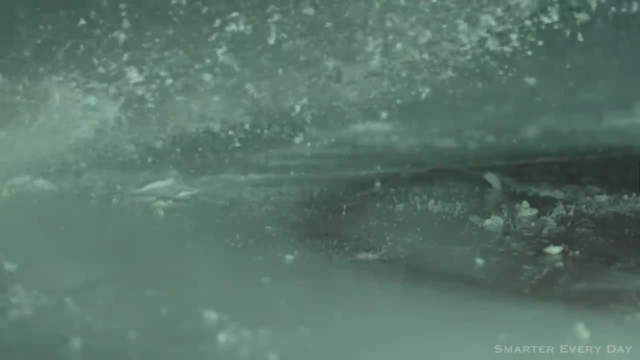 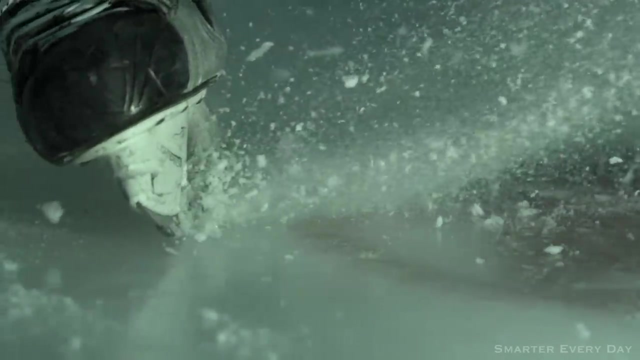 And he did it on the very first try. Can you imagine the math that's going on in his brain in order to automate this feedback loop? He's constantly sensing his deceleration And somehow his brain's converting that information to signals to control the angle of his skates and feather the exact amount of ice that he's shearing off. 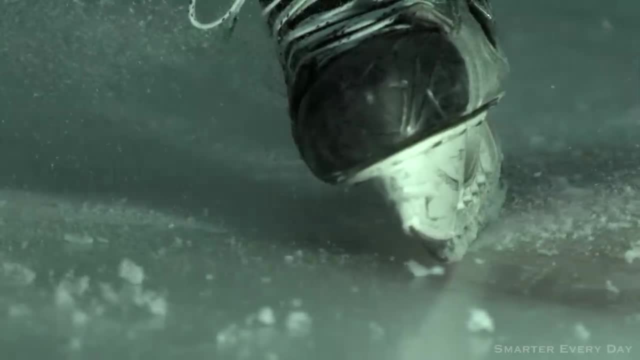 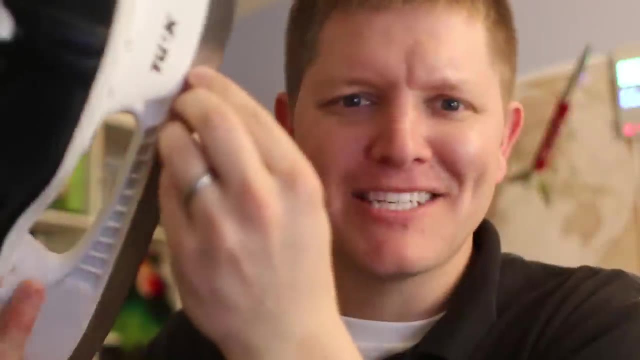 To complicate matters. he's got ice in between him and his target And he has to end it. He has to anticipate the total amount of impulse left in that ice so he can stop exactly where he wants to. Let's ask him to see if he can explain exactly what he's doing. 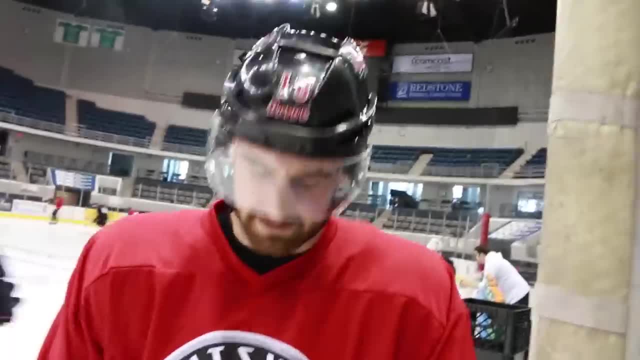 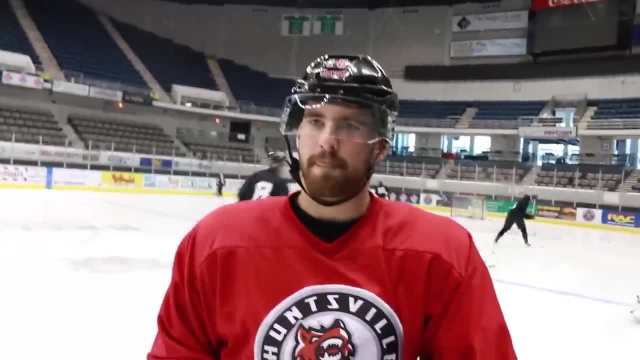 Because I'm pretty sure hockey players are physics geniuses. You ain't got to take your glove off, man Ben. thank you very much. Do you have any Like if you had to say anything about that hockey? stop. how exactly do you do it? 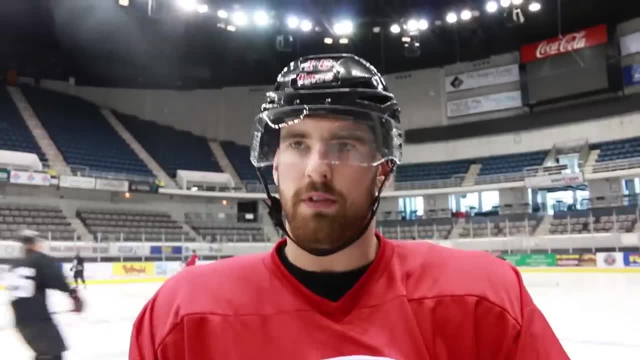 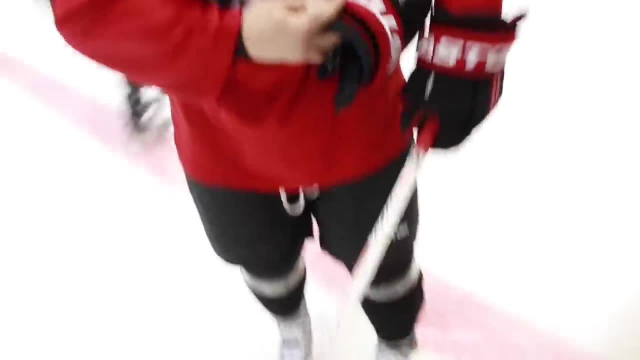 Are you? Well, you're just trying to find the balance Because you have two, There's two edges of the skate plate, So you want to find that inside edge. You know if you, If you get over the top with your outside edge, you go over. 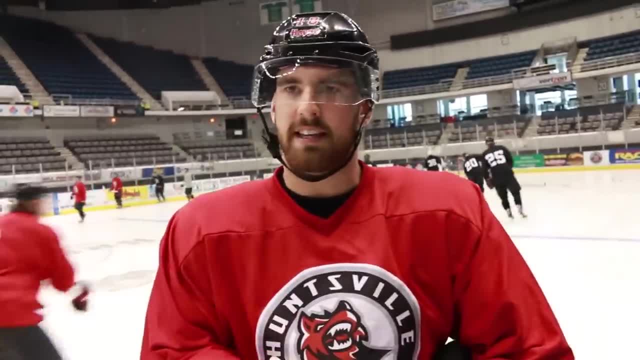 You're trying to find that edge on the ice and just shave and find the edge, Just the inside right. So, like a noob, somebody that's just learned how to do that, would they just chatter across the ice? Yeah, absolutely. 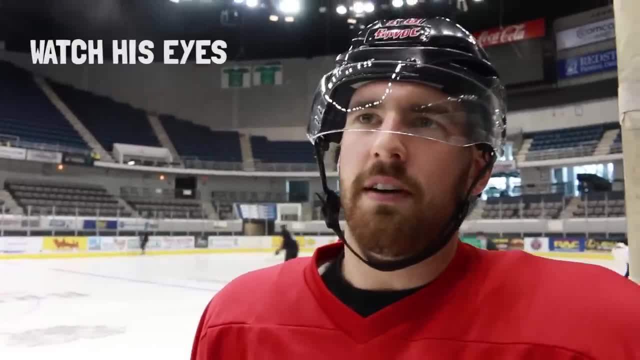 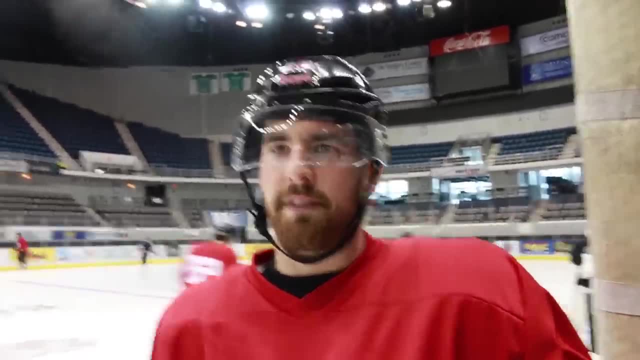 I mean, I started playing when I was like three years old, So maybe by the time I was like six I could stop. Yeah, You know So a couple of years. but like Did you just hit that puck without looking? 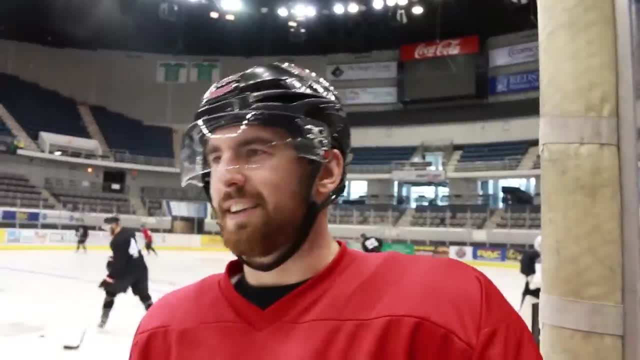 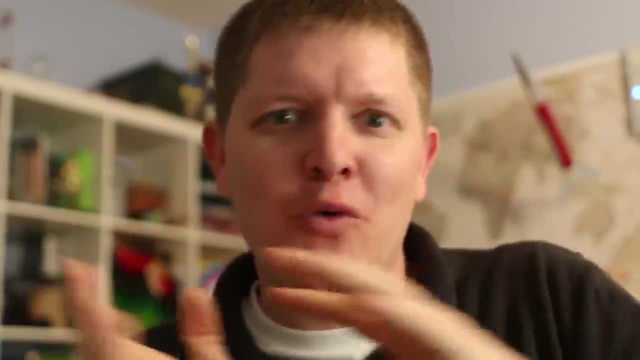 Yeah, He just hit a puck and you hit it without looking And then I saw it. Yep, I'm right, They're geniuses. So if we want grip for a hockey blade, we don't want it for a speed skate, right? 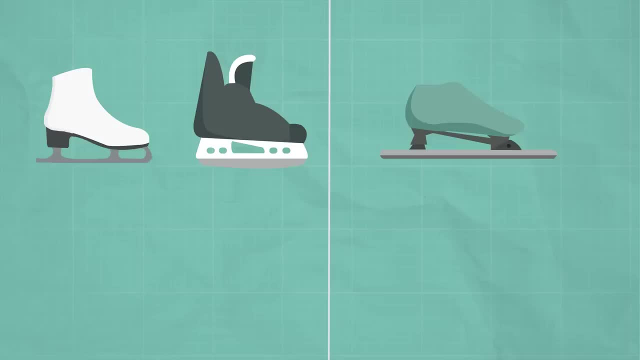 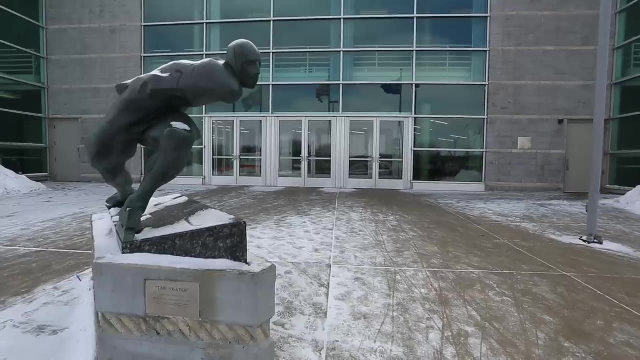 Which might explain why speed skaters are always falling. This was counterintuitive to me, but the bottom of a speed skate isn't pointy. It's actually a flat, sharp, 90-degree angle To see speed skaters in action. let's go to the Pettit National Ice Center in Milwaukee. 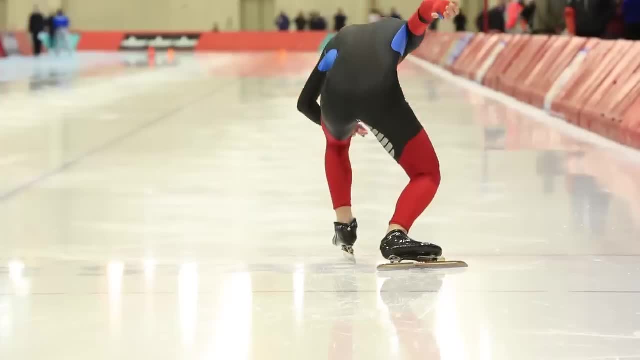 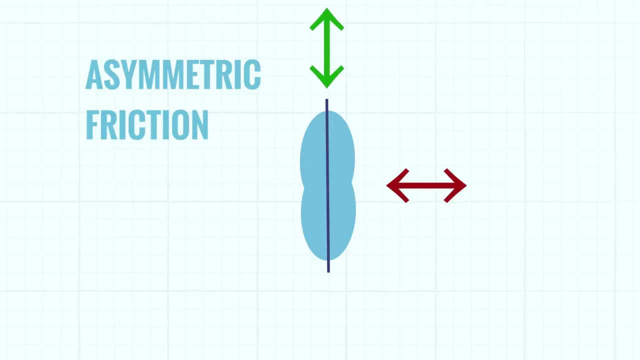 and check out the US Junior Long Track Championships. Okay, look at how the skater starts off the line. You see that open stance. They do this because ice skate friction is asymmetrical. They glide easily going forward, but they dig in on the sides. 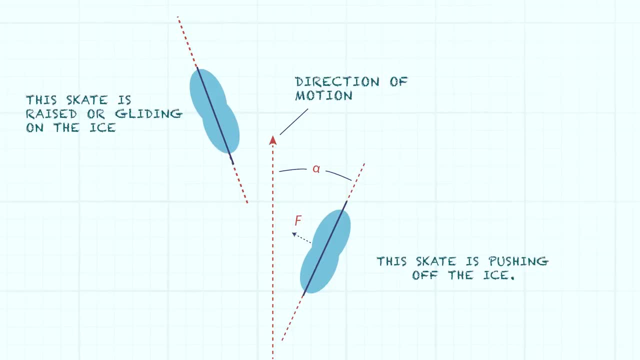 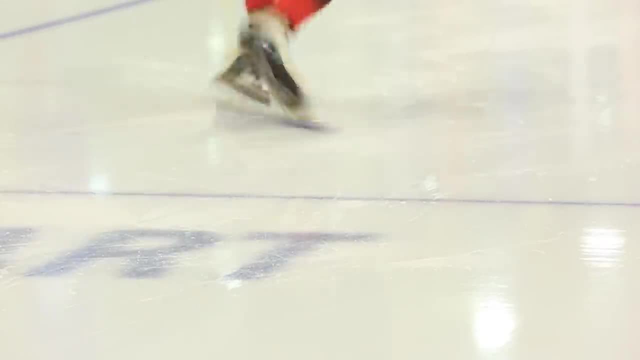 So to propel themselves, skaters have to push off the sides of the blade. The larger this angle alpha is, the harder they can push. That's why they line up with their foot at almost a 90-degree angle to the direction of skating. 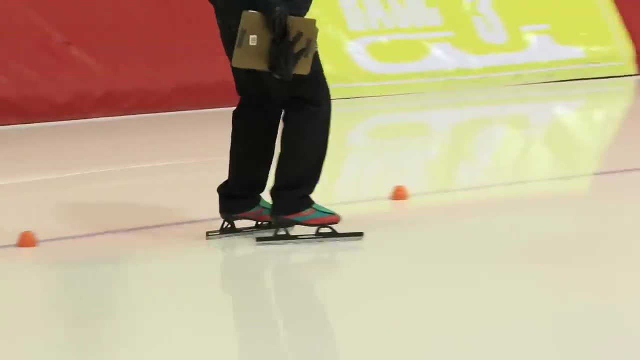 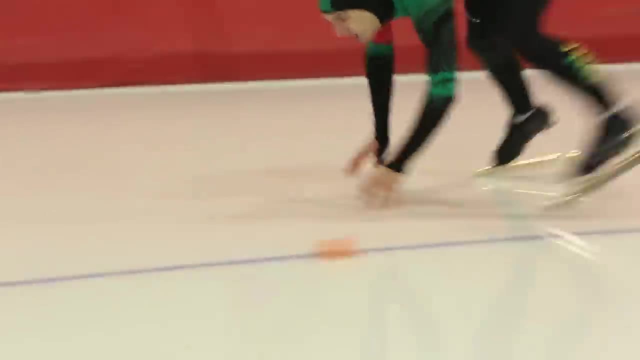 Speed skates are flat, which means each individual stride has to be perfectly level. when the foot hits the ice, This can be a problem because when you extend your ankle, the blade tries to come up off the ice. The solution to this is called a clap skate. 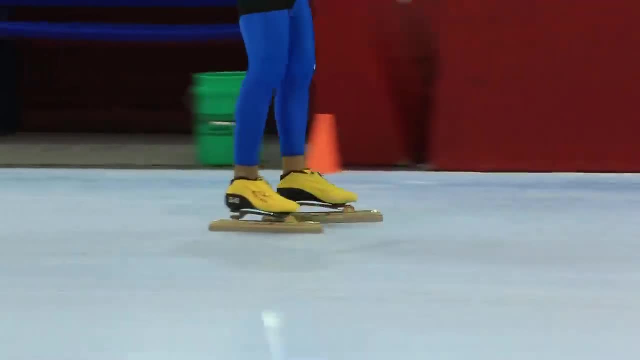 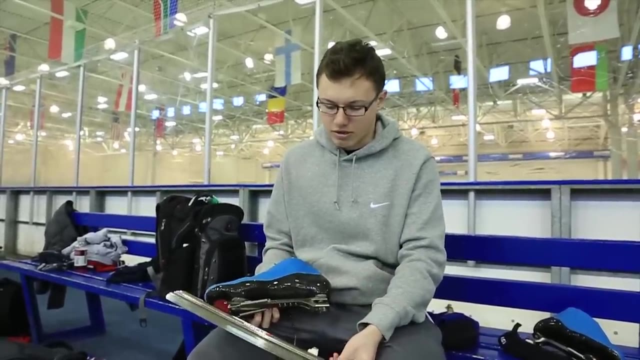 Clap skates allow a long track skater to keep their blade on the ice longer into the stride. I'll let Adam explain. The clap starts to come out like this Once they pick their skate up. it just kind of flies back like that. 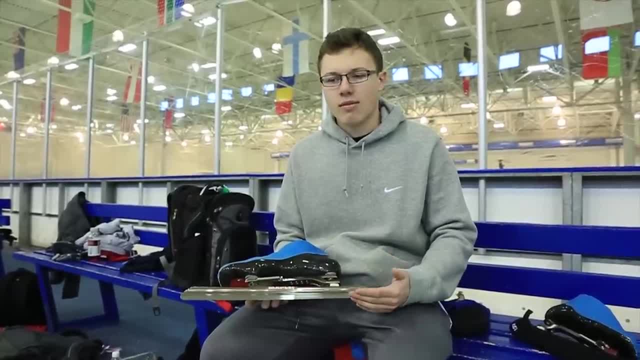 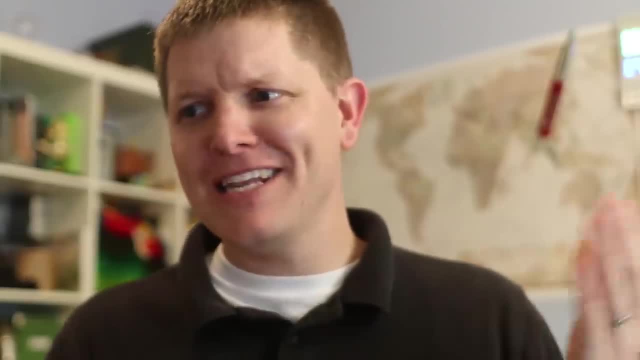 And so that extra push that makes the clap gives you a lot more contact on the ice, And so you can get a lot more power. All this talk about ice skating, and we didn't even explain why it's slippery in the first place. 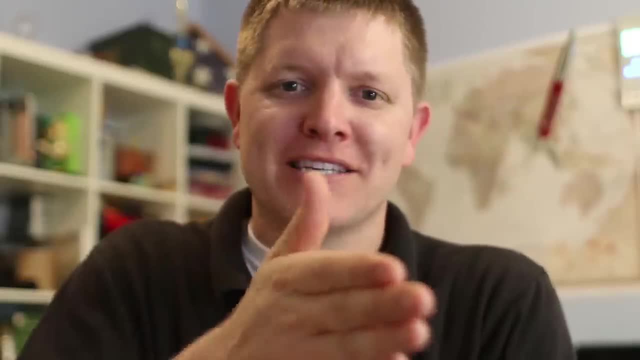 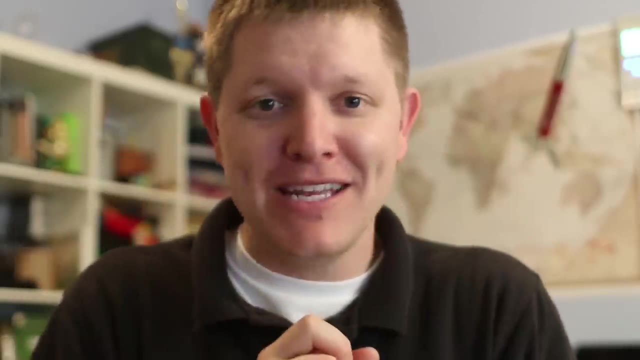 So there's this thing called friction melting. If you're moving something along ice, it creates this really thin layer of water, Think like nanometers thick. That is why you can slip on ice so easily. The coefficient of friction can be defined by this equation.